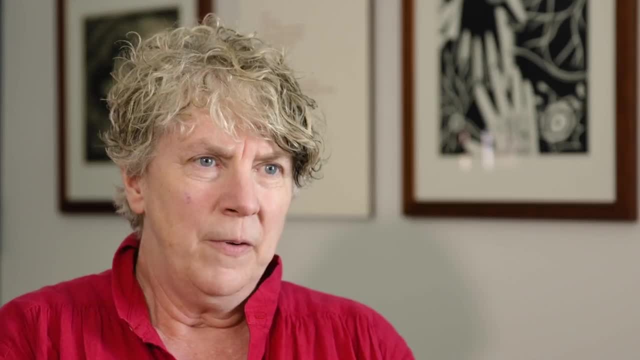 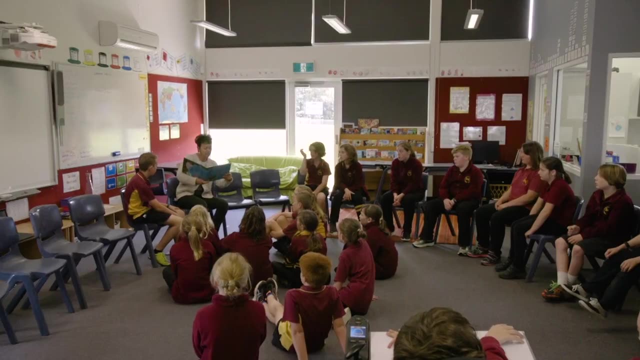 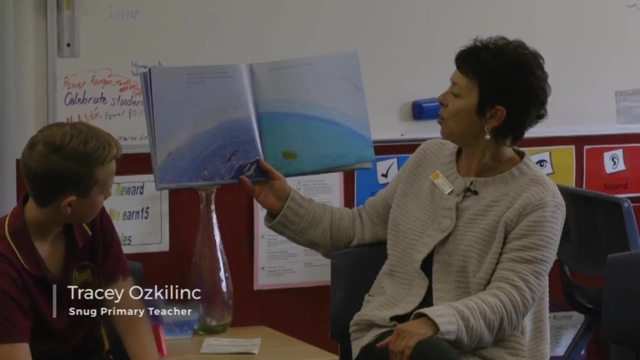 And the principle is that anybody can have a voice, their voice is heard, their voice is respected and other people can hear that voice. and yet they don't agree necessarily, and they explain why they don't agree. The class might be exposed to a question or they may look together at a book. 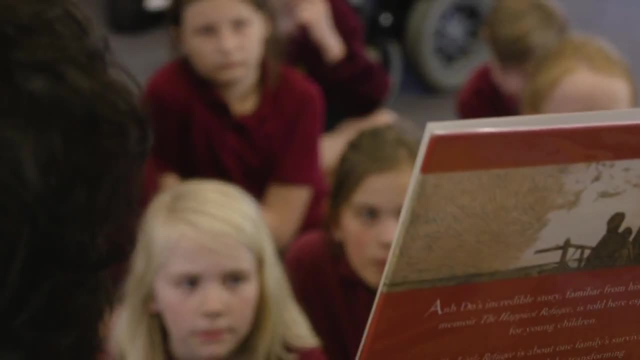 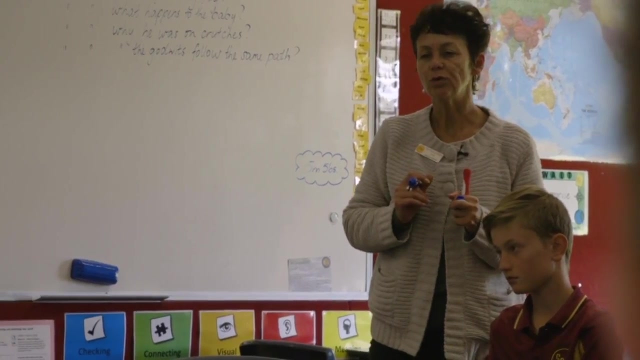 And a short book is often a very good book because it helps to keep the focus That inspires the children in the class to then ask a question of that. The great part about this is that the questions are coming from the students, not from the 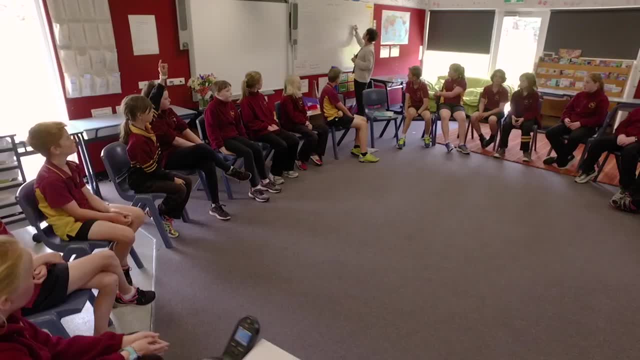 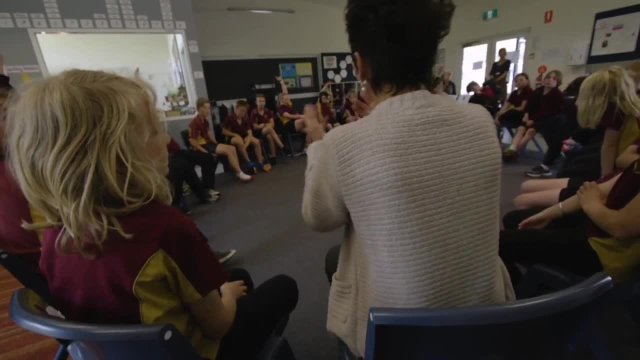 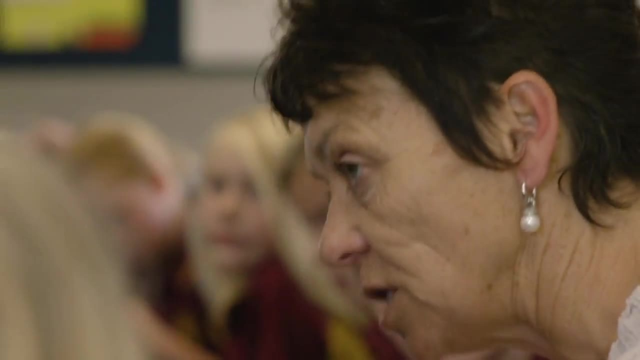 teacher. The teacher can put their own question in if they wish, but it's subject to the same straw vote as everybody else. It's not about going around the class and making sure everybody comes up with a question. It's really. is there something that you're interested in addressing? 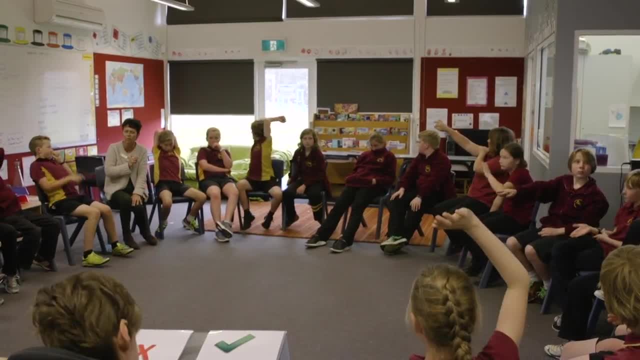 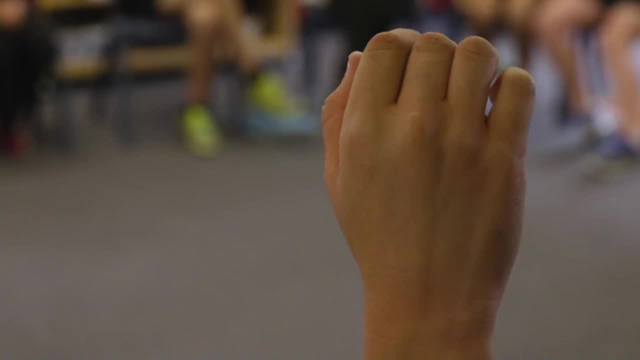 A few people agree with that. I'd like to hear from those people. Thank you. I'd like to hear from those people who disagree. The inquiry is about that one question. It's really important that we are respectful and accepting that people have different ideas. 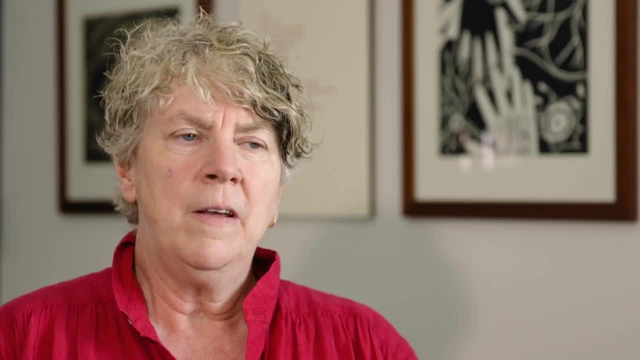 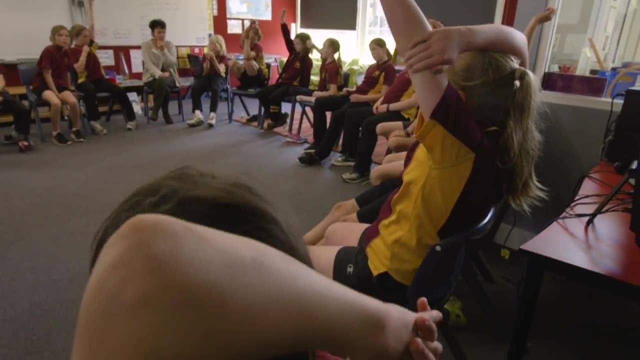 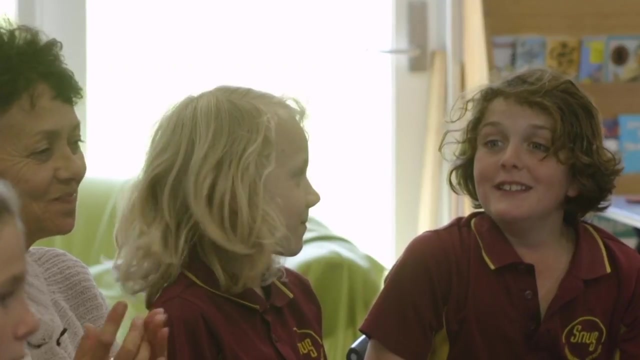 The conversation, on the one hand, is free flowing but, on the other hand, has a certain structure about it that is encouraging respect of everybody who has a voice, And that's the key part- is that it's a safe place for people to express their view. 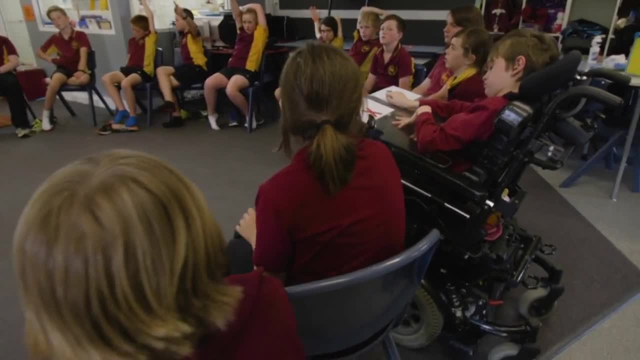 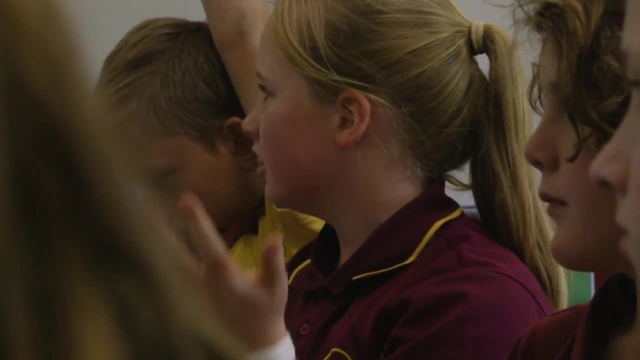 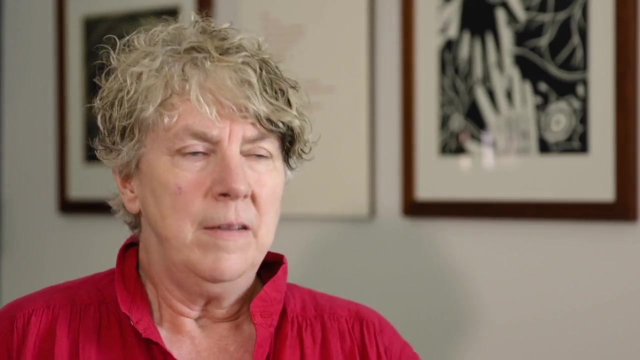 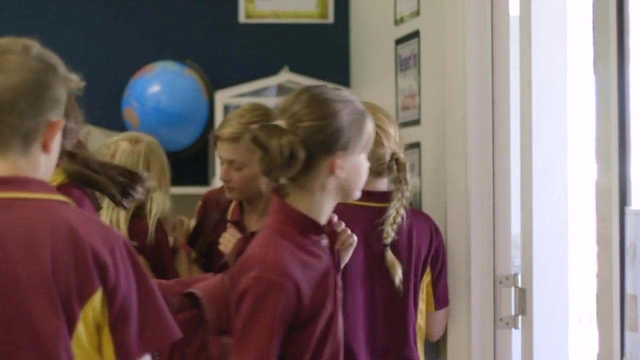 This activity can deepen as people become more comfortable and as the group understand the role that they can play. It's a practice rather than a task. It can be something that we can take time aside to develop a community of inquiry for that half hour period and then return and see how that might apply to other areas of. 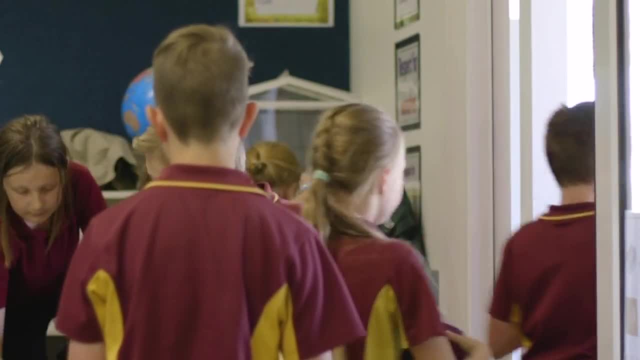